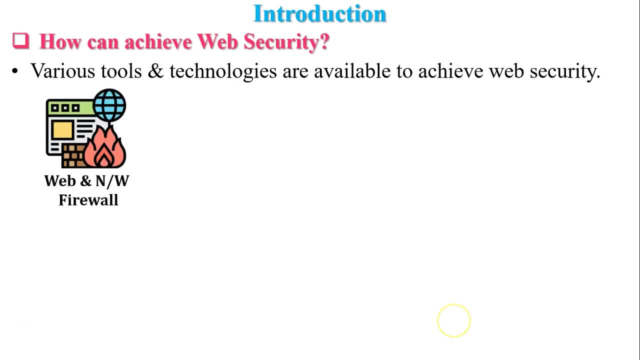 technology to achieve web security. The first one is web and network firewall. Web application firewall sets between your website server and the data connection. The purpose is to read every bit of data that passes through it and to protect your site. Network firewall is set between your network device and your. 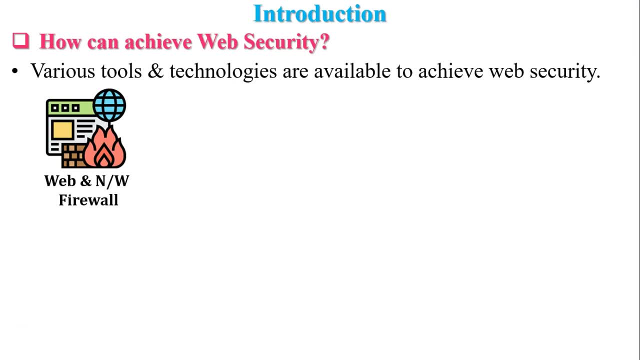 computer system. It is used to protect your network and your computer system. It is used to filter the incoming and outgoing data in the network. Web firewall: protect your website and network firewall: protect your network. The next one is keep your software up to date. If your website software or applications are not. 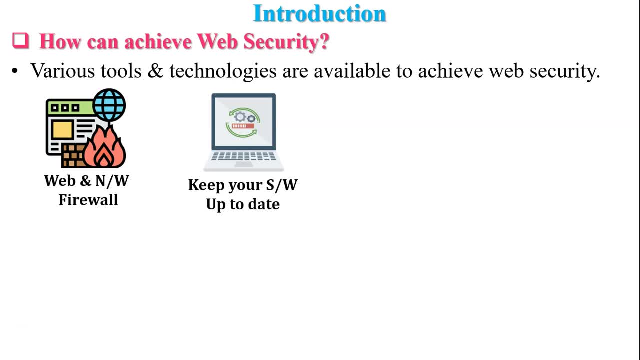 up to date, your site is not secure. Updates are vital to the health and security of your website. Take all software and plug-in update requests seriously. Also, use HTTPS and SSL certificate to secure your website. The backup, your data, Backup of your website regularly. You should maintain backups of. 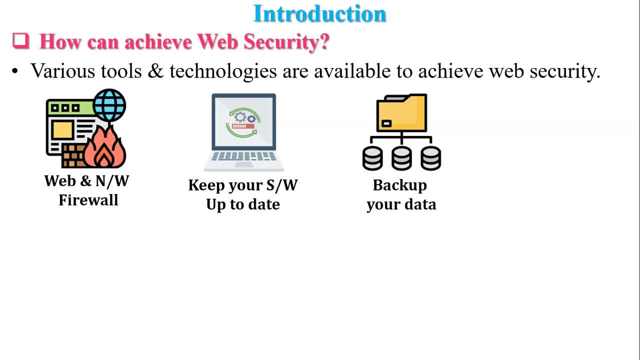 all your website files in case your site becomes inaccessible or your data is lost from the server. Next one is keep your website clean. Every databases, applications or plugins on your website is another possible point of entry for hackers. You should delete any files, databases or applications from your 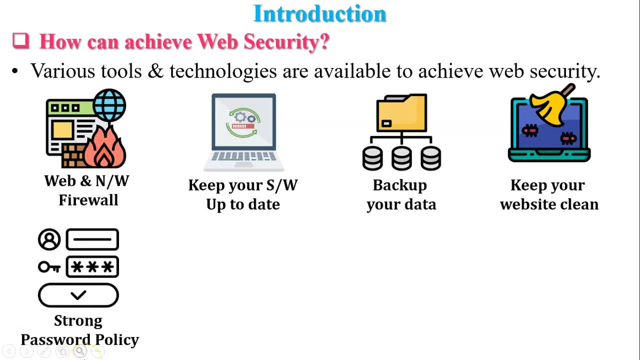 website that are no longer in use. Next one is strong passwords policy. It is important to use strong passwords to protect against root fault. Passwords should be complex, containing uppercase and lowercase letters, numbers and special characters. Your password should be at least 10. 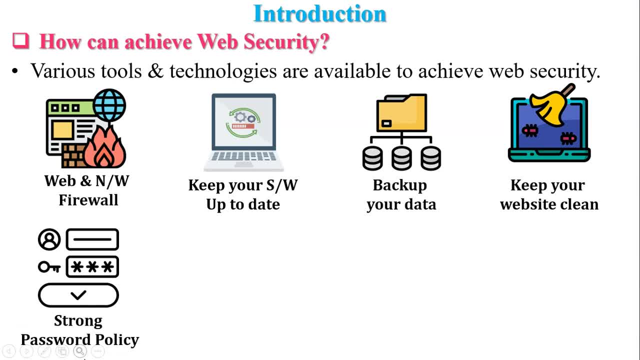 characters long. Also apply this policy with your organizations. The next one is password cracking tools. Password cracking tools help to restore the lost password. Whether you have forgot your password or your password has been hacked, A password cracking tool can help you recover your password. The next one is scan your website for 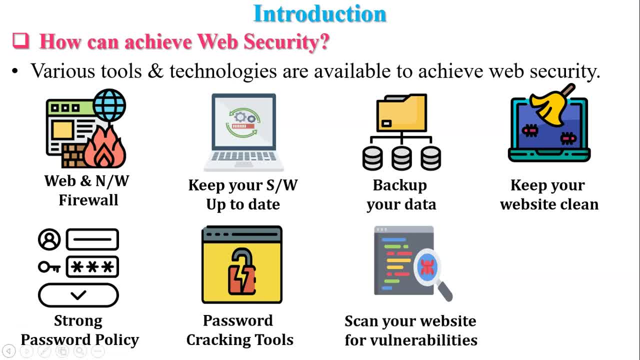 vulnerabilities. It is important to regularly perform web security scans to check for website and server vulnerabilities. Web security scans should be performed on a scheduled basis and after any changes or addition to your web components. And the last one is use antivirus. Antivirus software helps. 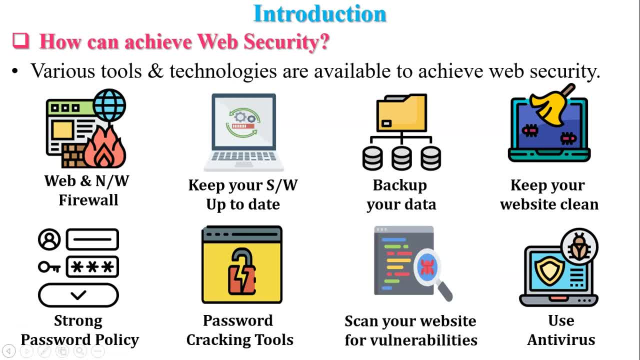 protect your computer against malwares and other incoming threats. Antivirus software looks at data like web pages, files, software applications which are traveling over the network to your devices. Antivirus searches for known threats and monitors the behavior of all programs and flagging suspicious. 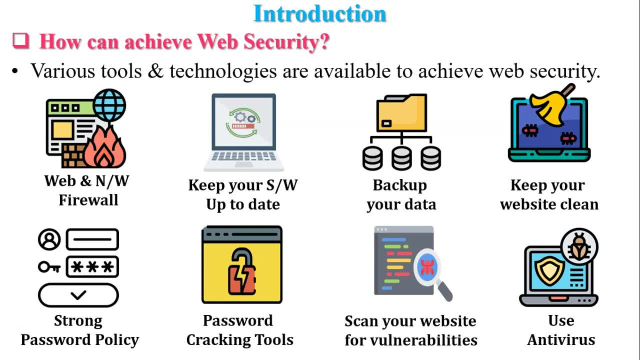 behavior. So these are some examples of tools and technologies to achieve web security. Nowadays, many more tools and technologies are also available on Internet. Next, what are web security threats? Web security threats are very common in the internet. In the internet, there are many ways. 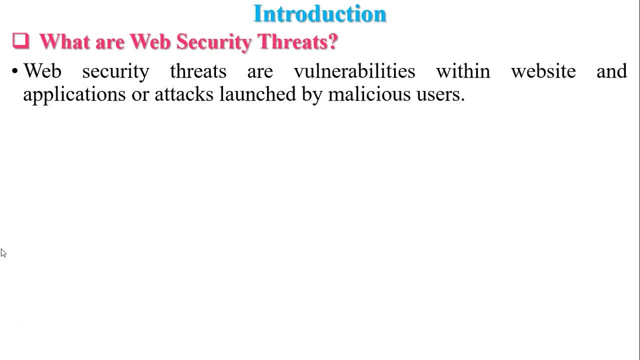 Web security threats are vulnerabilities within websites and applications or attacks launched by malicious users. Web security threats are designed to breach security of websites or applications. So here I am discuss some of the example of web security threats. The first one is modification of message. 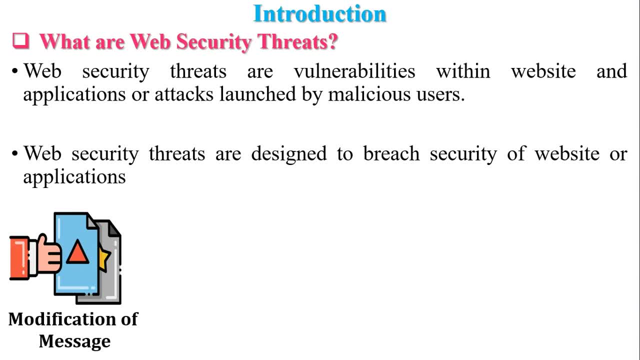 Message should not be altered during the transmission, So it is called: there is no integrity in the message. If message has been changed during the transmission, it is also called as data breach. It means some confidential and sensitive information gets exposed, So it is one kind of biggest threat in the internet. 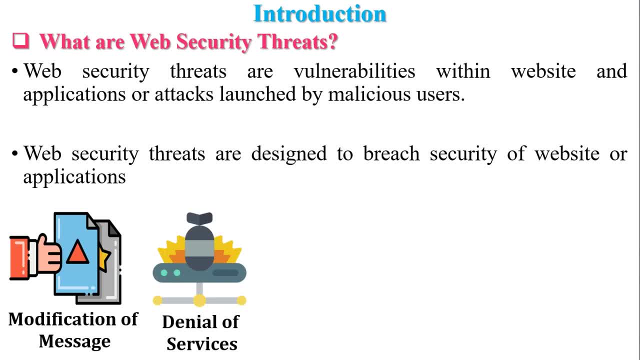 Next, Denial of services. It is also known as DDoS. Denial of services is a web security threat that involves attackers flooding servers with large volume of internet traffic to disrupt service and take website offline. Website is inaccessible for other users. The next example of threat is phishing. 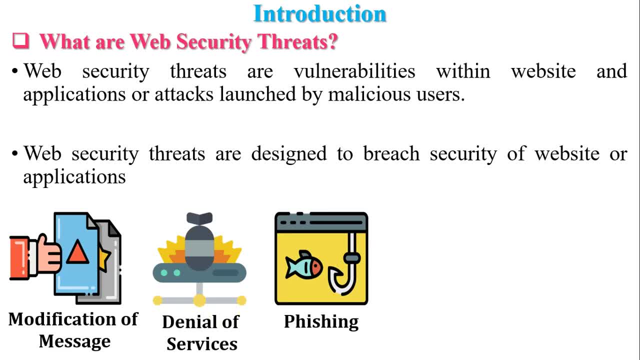 Phishing attack targeting users through email, text message or social media messaging sites. Attackers impersonate as a real user or real website, So users can trust that and click on given link and provide the sensitive information, like account number, credit or debit card data and login credentials. 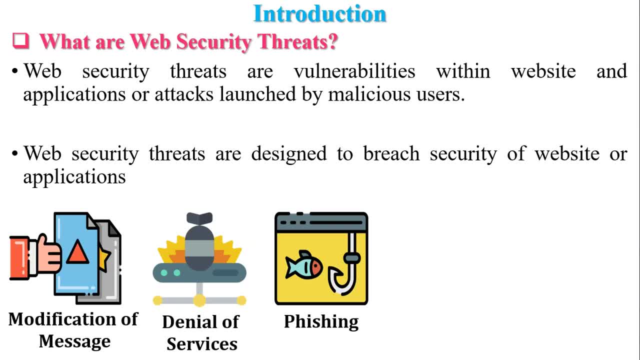 Through the phishing attack, user can lost their money as well as sensitive information. The another example of web security threat is SQL injection. SQL stands for Structural Injection. SQL is used to search and query databases. Nowadays, phishing and SQL injection is a most popular web security threats. 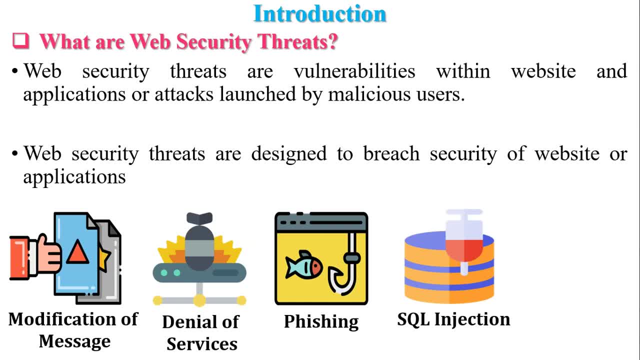 SQL injection is the placement of malicious code in SQL statement via web page input. Using SQL injection, hacker can retrieve user credentials and some sensitive information through the SQL query in web pages. Another example of web security threats is Malwares. Malwares stands for Malicious Search. 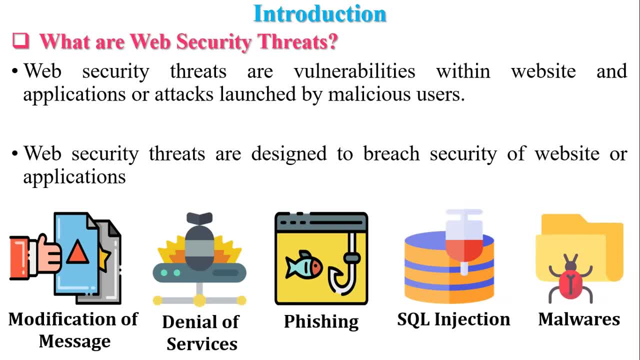 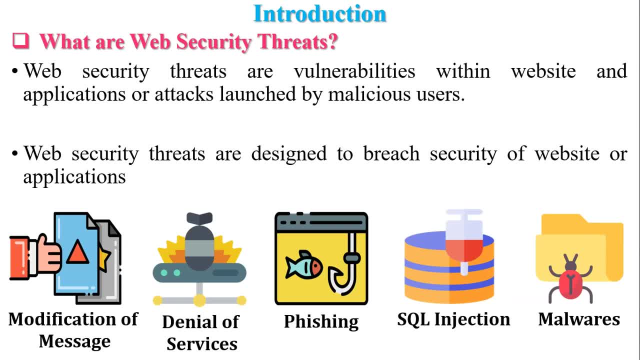 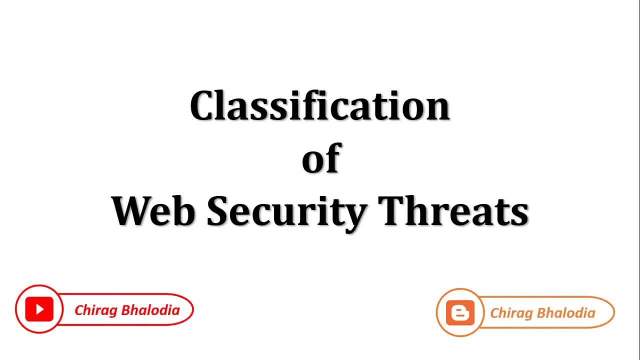 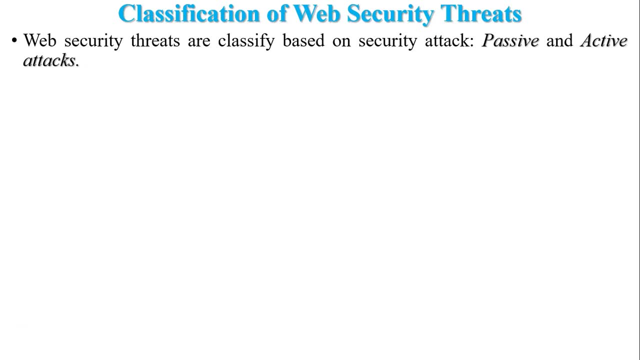 or conducts virtual any behavior an attacker wants. So these are the web security threats which is most popular nowadays. Next classification of web security threats. Basically, web security threats are classified based on security attack. It may be a passive or active attack. Another way to classify web security threats is in terms of location. 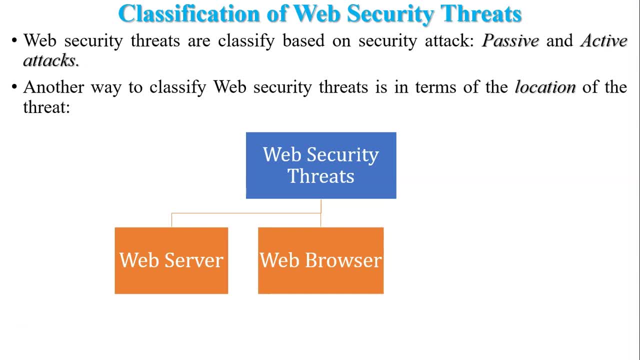 The first one is web servers, The second one is web browsers And the third one is network traffic. Web server and web browser falls into the category of system security, And network traffic is under web security. So in this video I have discussed about web security threats. 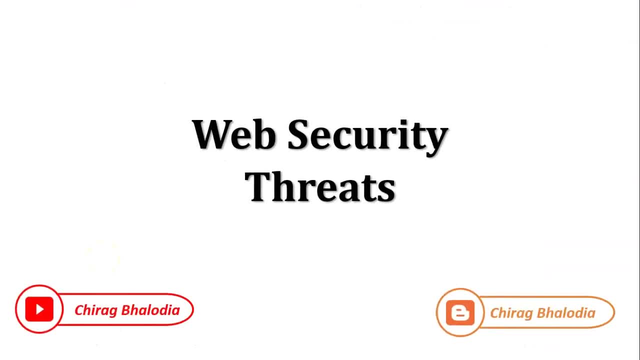 Now discuss web security threats. Here we have discussed web security threats based on security goals. If you want to learn about web security threats, you need to know about web security threats. If you want to learn about security goals, then click on above i button. 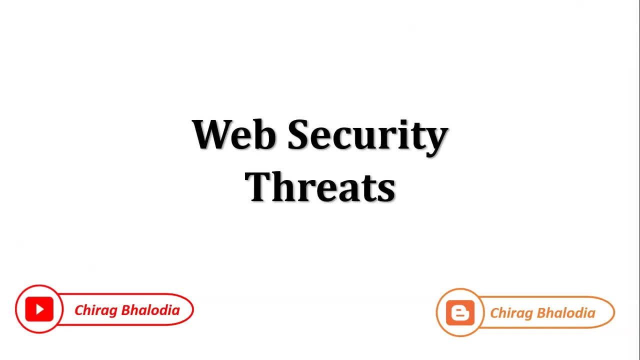 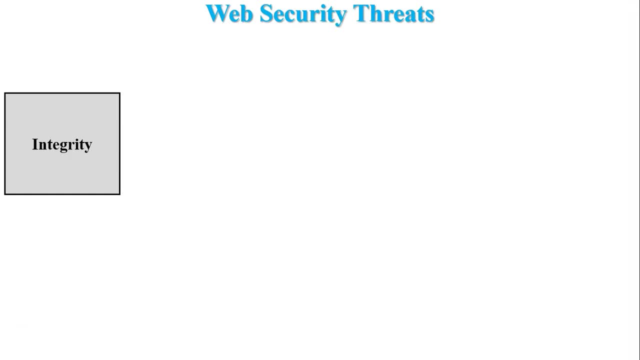 Also discuss consequences and countermeasures of web security threats. So let's start with integrity. Integrity means message should not be altered during the transmission. If message is altered, it means the integrity is broken. So how threats break the integrity? The first one is modification of user data. 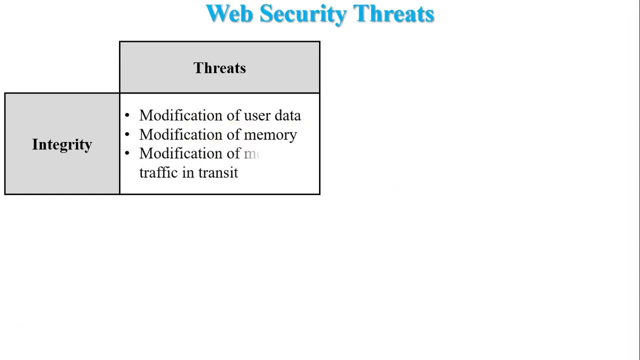 The other way is modification of memory, And the other method is modification of message traffic, Intrinsic after break the integrity. there are so many consequences. the first one is loss of information, the second one is Compromise of machine and the third one is vulnerability to all other threats. So here loss of information means 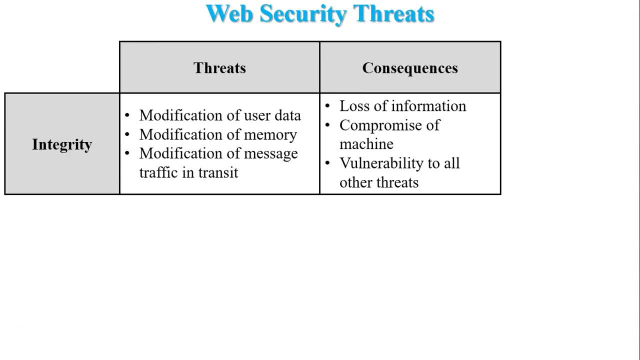 Modification of users data. the compromise of machine is modification of memory. So integrity is great. It means the vulnerability to all other threats are increased. So how to counter this threats? using the cryptographic checksums. So here there is one question: What is cryptographic checksum? 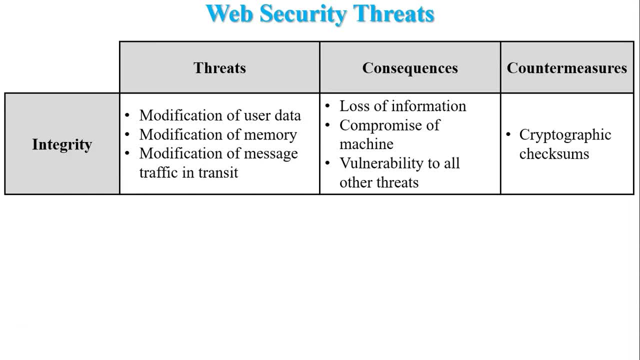 Before sender sending a data, generate a checksum and that checksum is Append with message and send to the receiver. at the receiver and receiver receive that message and generate a checksum. if receivers checksum and Appended checksum which was generated by the sender, if both are same, it means there is no integrity in the message and 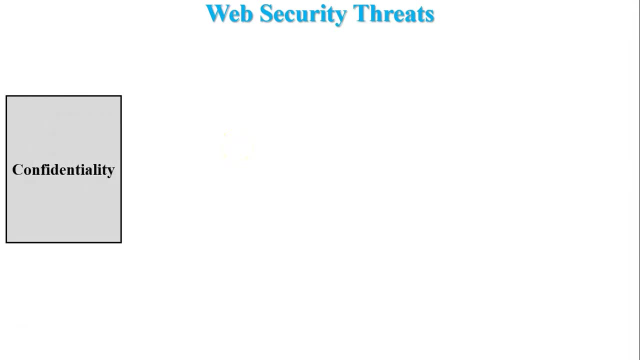 Receiver accept that message. the next one is confidentiality. Confidentiality means the message should be known by only sender and receiver. So there are some threats to destroy the confidentiality. The first one is us dropping on the internet. us dropping means someone listen your conversation on internet But you don't know about that. 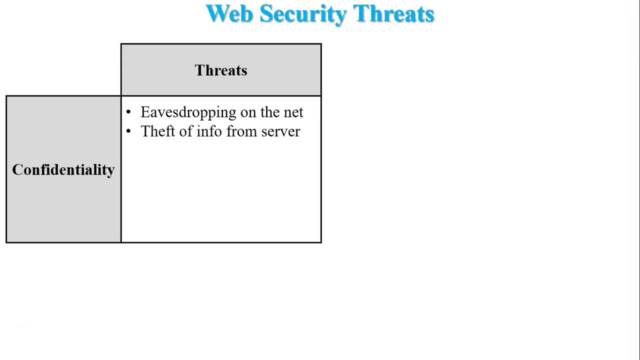 The next one is theft of information from the server. The another one is theft of data from client. The next one is information about network configuration. if attacker or hacker can get the information about network configuration, Then they can capture the message from your network and destroy the confidentiality of data. 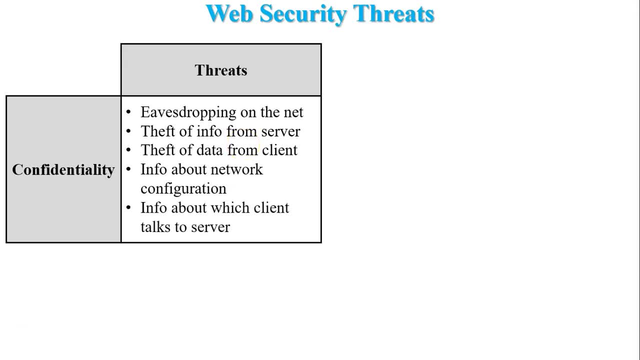 The next one is information about which client talks to server. So this is one kind of passive attack. if confidentiality is brave, then the consequences are loss of information. So here, loss of information means attacker and hacker can get all the information of client From the server, as well as capture the messages between server and client will communicate. 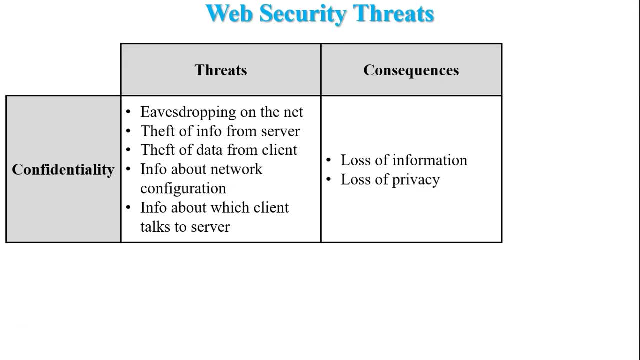 Another consequences is loss of privacy. It means when server and client will communicate. at that time attacker or hacker can capture that message and know the secret Information or messages from the communication. that is called loss of privacy of particular message. So how to protect this threat? using the encryption and use of web proxies, or you can use private VPN in your. 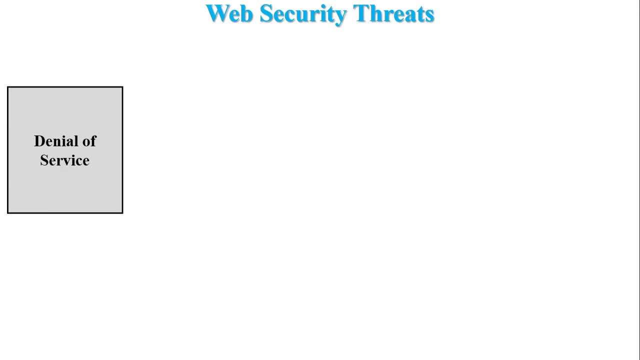 organization. The next one is denial of services. Denial of services means interruption in an authorized user to access web services or network. It is called denial of services. the threats to denial of services are: first one is killing of user threats When the communication between server and client is going on. at that time server and client are disconnected. 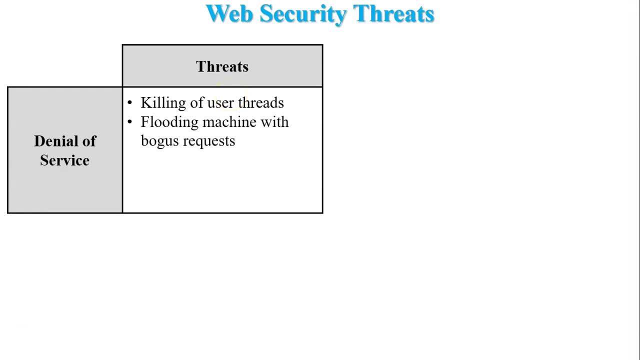 It is called killing of user threats. The next one is flooding machine with bogus requests. So it means attacker and hacker Can access the server and continuously send a bogus request to the server. So after sometimes server is full of requests and server goes down. next, filling of disk or memory. 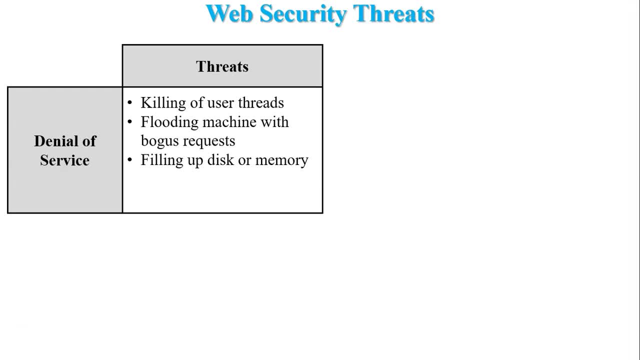 if number of requests are sent by the Attacker or hacker. at that time the server's disk or memory is full. So it means server is set down after some time and disconnected from the network. The next one is isolating machine by DNS attempts if any loopholes in 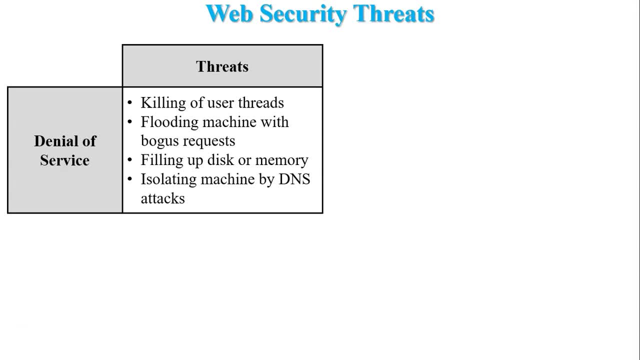 DNS. then attacker can attack DNS tunneling, DNS poofing in, DNS flood attack and the services of the server is denied. the consequences of the denial of services is Disruptive, so user cannot access the server, So it is annoying to the user. and the next one is prevent user from getting work done. 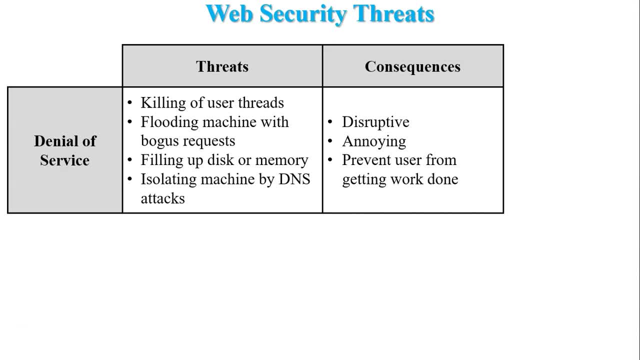 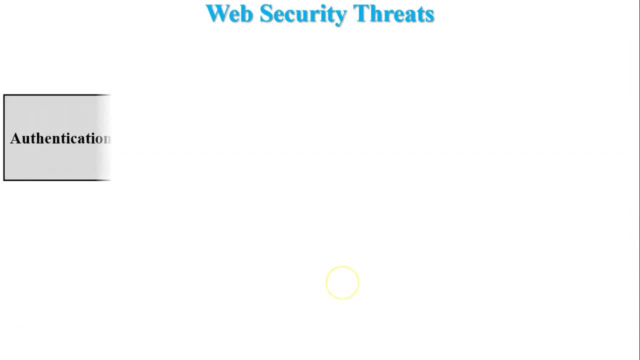 It means user cannot access any data from particular server and cannot submit any data to the server. So denial of services is difficult to prevent. The next one is authentication. Authentication is a process to verify users identity. So the threats are impersonation of legitimate users. Impersonation means fake website or fake user. act as a real user or real website. 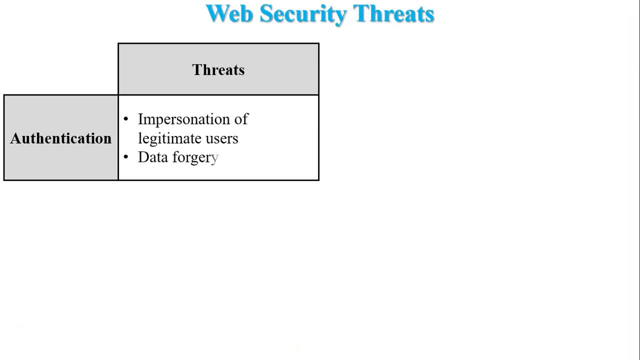 So it is one kind of phishing attack. The next one is data forgery. Data forgery means some fake user act as a real user and send some link to the user so user can click on that link and Give the information. so it means attacker or hacker can get the users information. So it is called data forgery. 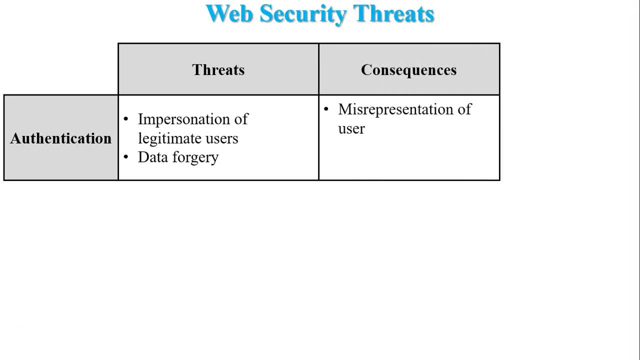 so the consequences are misrepresentation of user because of impersonation of legitimate users, and The next one is belief that false information is valid. So how to protect this? threats to achieve the authentication cryptographic techniques are hash function message authentication code, digital signature and digital certificates. next, there are the comparison of web security. 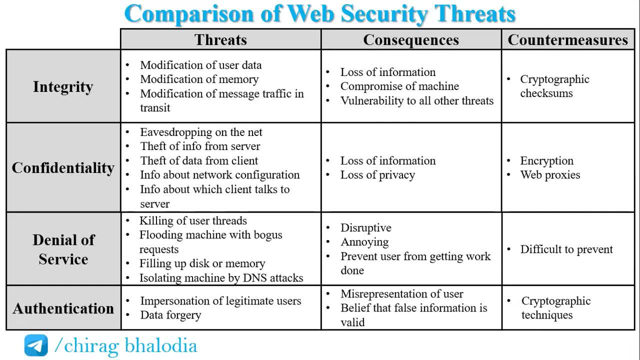 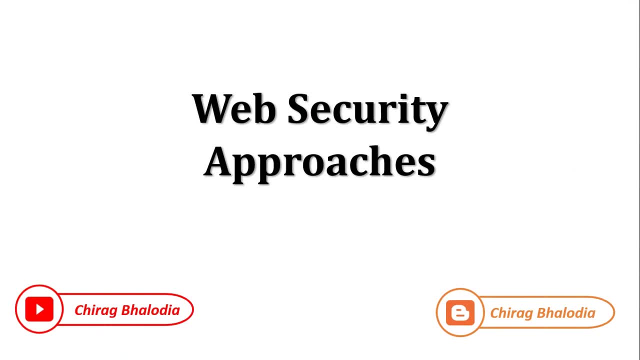 Threats. for further discussion, you can join my telegram group, Chirag Balodia. link is given in description and this video material is available on my blog, Chirag Balodia dot com. Let's discuss web security approaches. a number of approaches to providing web security are possible. 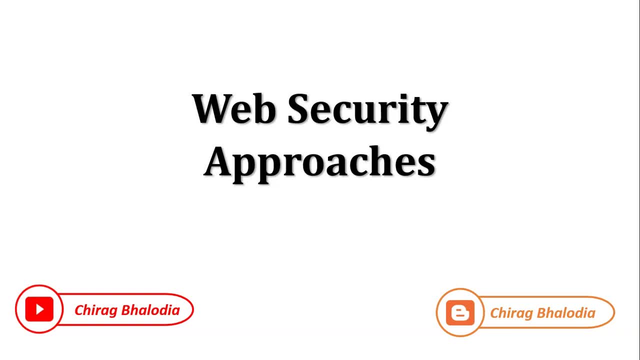 The various approaches that have been considered are similar in the services and the mechanisms that they are used, But it may be differ with respect to their scope of applicability and the relative location Within the TCP IP protocol step. so here we are: discuss web security approaches with reference to TCP IP protocol state. 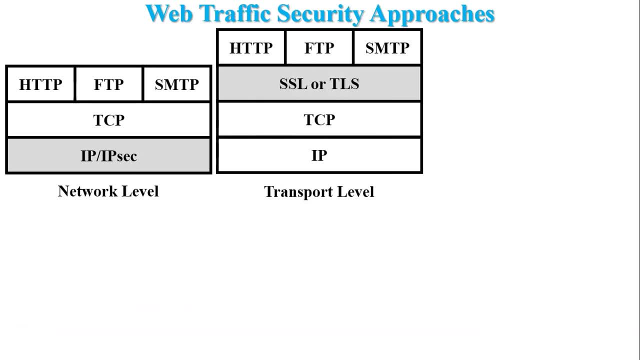 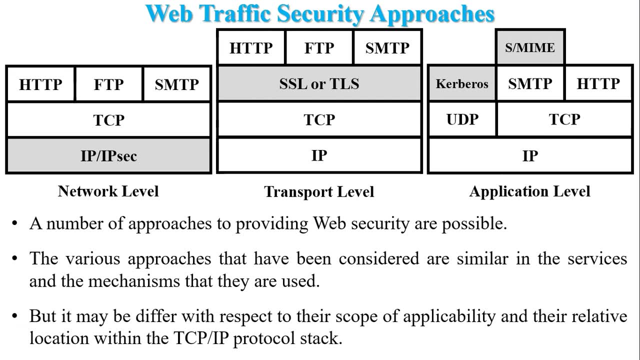 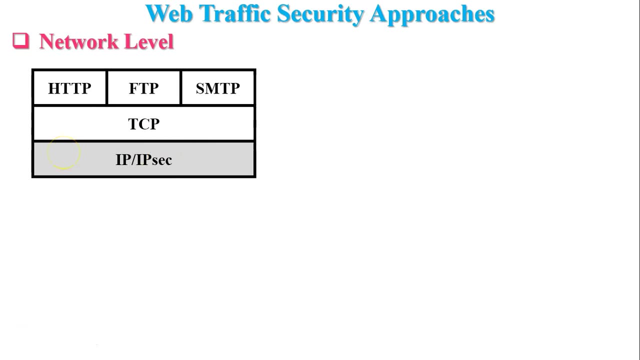 So first one is network level, the second one is transport level and the third one is application level. So now discuss all these three security approaches one by one in detail. The first one is network level. in network level, web security can be achieved through IP address, Because only internet protocol is used in network layer. 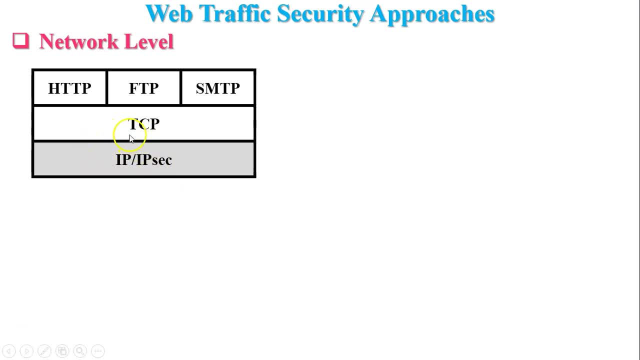 So web security is based on Internet protocol is called as IP sec. It is called IP security. the advantage of IP sec is that it is transparent to end-users and Applications and provide a general-purpose solution. the another advantage of IP sec is filtering capability, So that only selected traffic need incur the overhead of IP security processing. 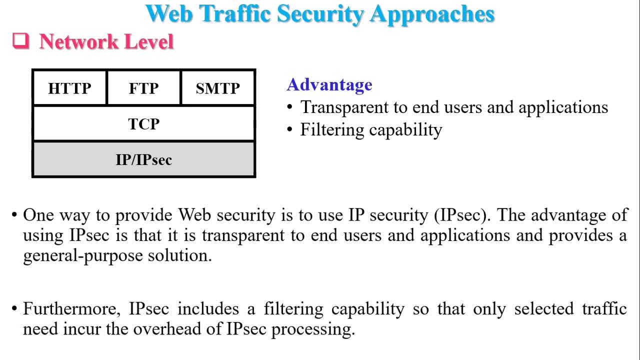 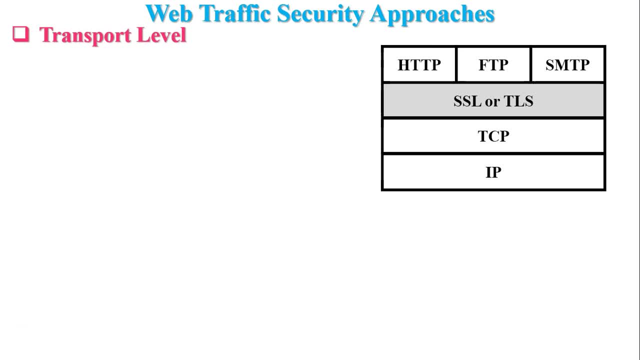 So what I have discussed in network level is written over here in this slide. You can read from this slide. The next one is transport level security. In transport level security the general-purpose solution is implemented: the security just above the TCP. The example of this approach is SSL and TLS. 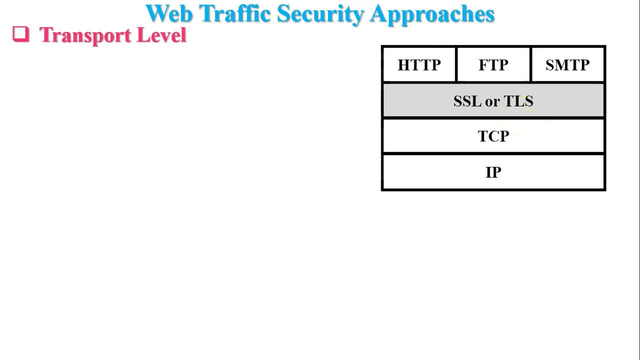 SSL stands for secure socket layer and TLS stand for transport layer. security advantage of SSL is transparent to application Because transport layer is provide process to process delivery in the network. another advantage of SSL can be embedded in specific packages. for example, Netscape and Internet Explorer is equipped with SSL and most browsers have implemented the protocol. 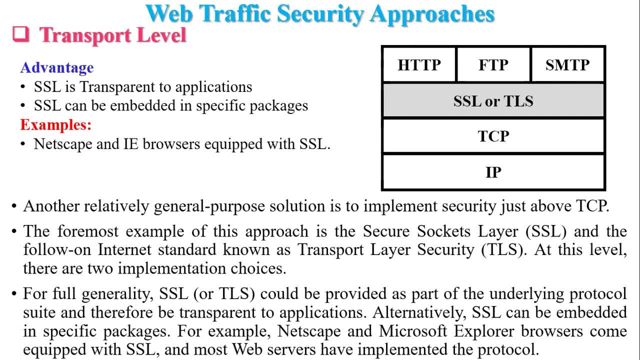 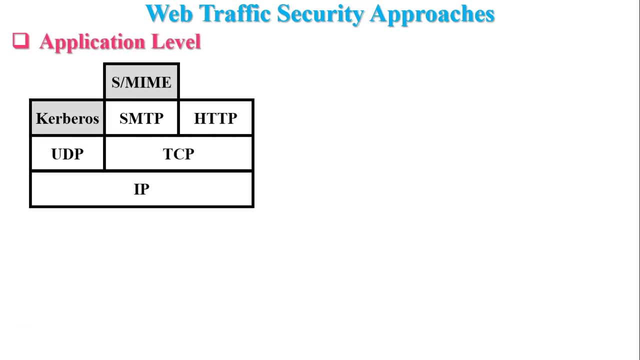 So what I have discussed in transport layer security is written in this slide. You can read from this slide. Next one is application level security. in application level security It provides application specific security services that are embedded within particular application. For example, you are sending a mail with multimedia file. 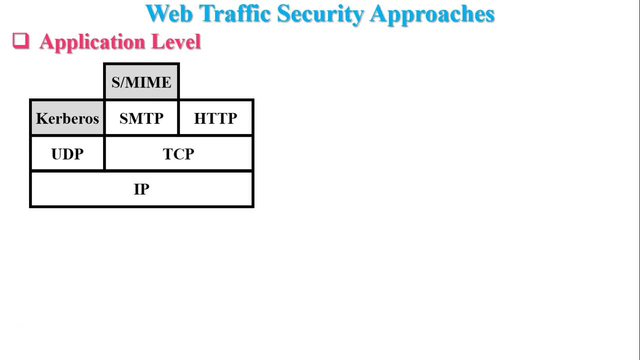 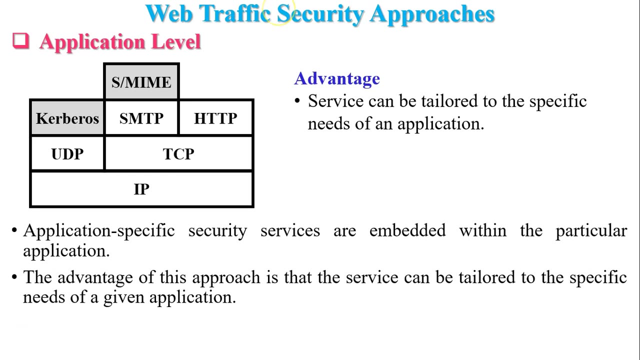 it provides that security based on SMTP and MIME protocol. Advantage of this approach is service can be tailored to the specific needs of an application. So what I have discussed in application level is written in this slide So you can read from this slide. For further query, you can join my telegram group, Chirag Balodia. The link is given in description.